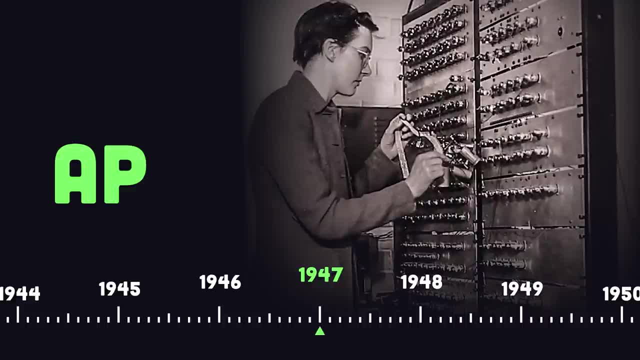 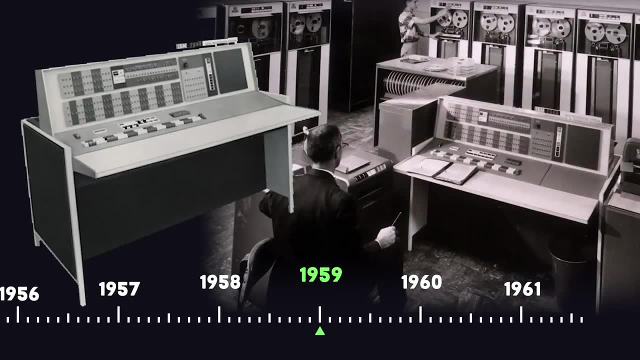 created by Kathleen Booth in 1947 for the all-purpose electronic computer. Over the next decade it evolved into many different formats to power the supercomputers of the day, like the IBM 7090, which had a $20 million price tag in today's dollars. Writing code in assembly was standard. 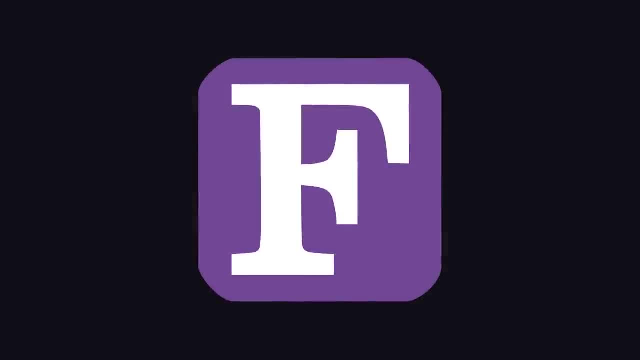 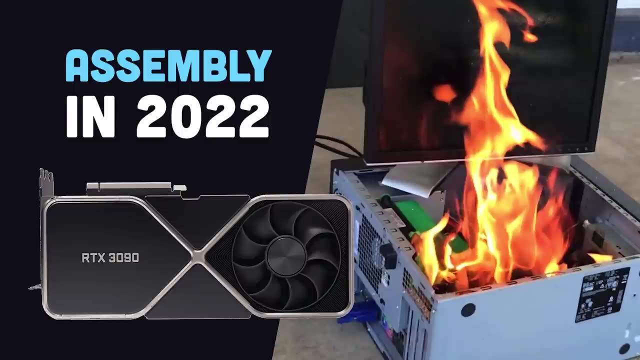 until the emergence of high-level languages like Fortran a few years later. However, assembly is still used today for direct access to the bare-metal hardware and to address low-level performance issues, often on device drivers and embedded systems, and it's also used to run native. 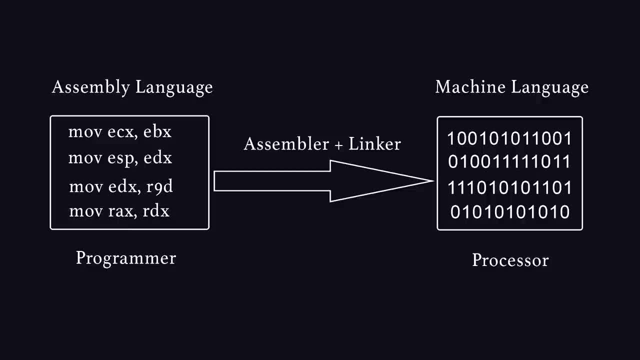 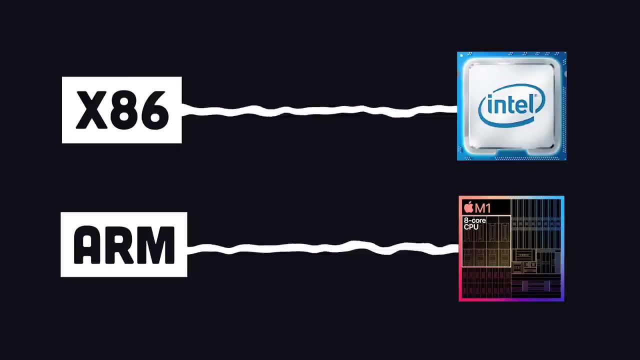 software in a web browser via WebAssembly. What's tricky is that each assembly language only works on a specific CPU architecture, like ARM for Apple, Silicon and Raspberry Pi, or x86 for Intel chips. To get started, you'll first need an assembler like the NetWide Assembler for x86 chips In. 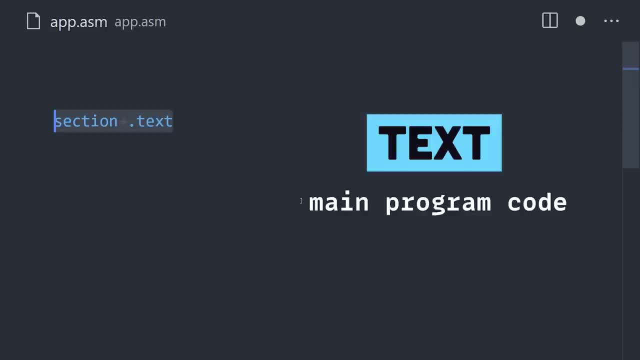 the NetWide Assembler. the assembly program is divided into three sections. The text section contains the actual logic for the program. By convention, it contains an entry point called start, which is where the code will start executing. Next we have the block starting. 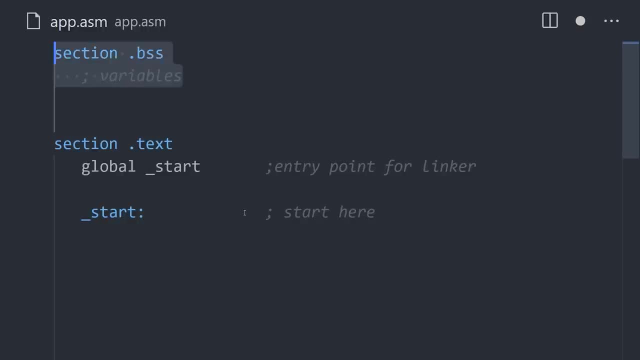 symbol section, which contains variables that might change throughout the lifecycle of the app. And finally, the data section is where we can initialize constants or data that does not change. To declare a constant like a string, we start with a label, then use db for define byte. 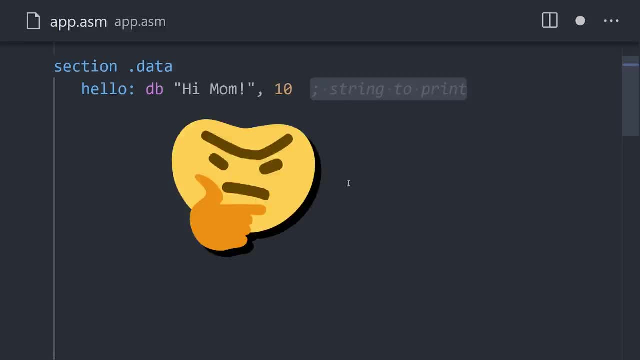 to place the hello world string into memory. By itself it doesn't do anything, and to print it will also need its length. We can use equate to convert a symbol into a constant. The dollar sign will subtract the current position from the hello label, providing the length of the string. And now? 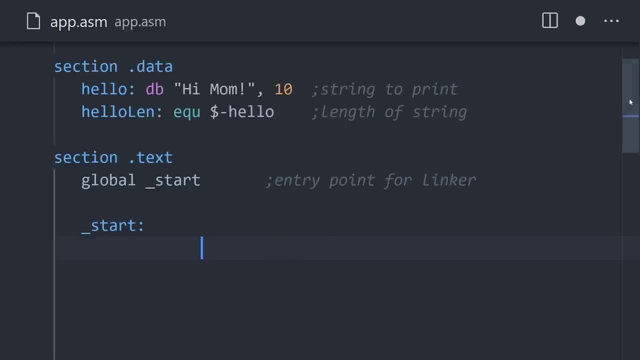 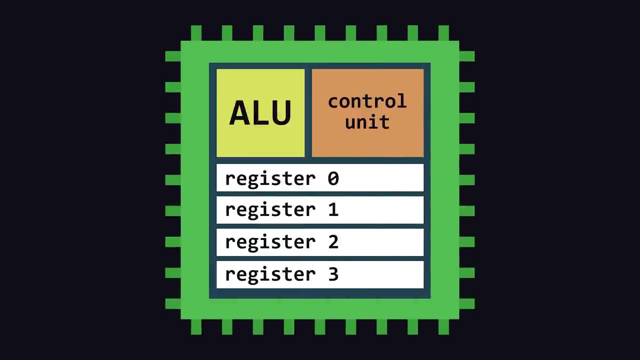 these constants can be referenced from the start label In the main program. each line of code contains an instruction along with one or more operands, and there are hundreds of instructions built into the language. Now to perform operations quickly, the CPU has a limited number of registers. 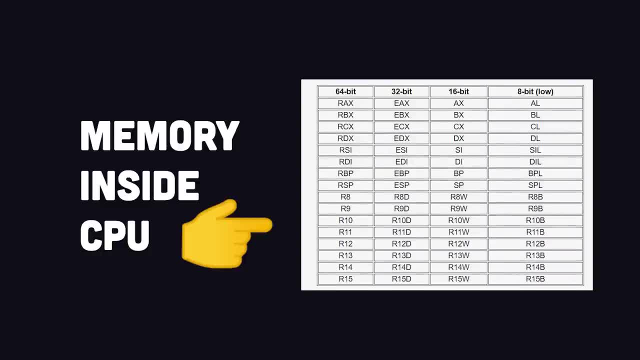 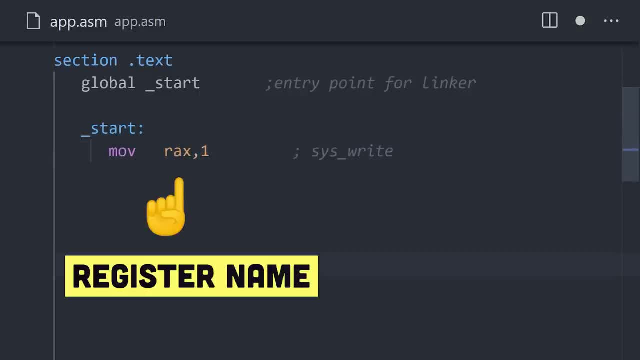 which are like 64-bit chunks of memory built directly into the CPU instead of the RAM. We can insert data into a register with the move instruction by providing operations that are operands for the register name and the data to store there. In this case, number 1 is used because 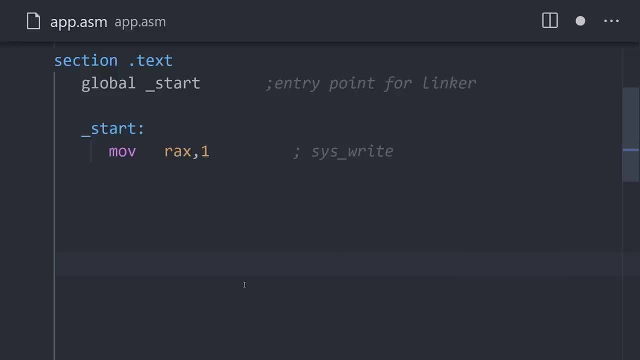 it corresponds to system write on Linux. Next, we need to tell the system where to write, in which case we will move 1 into the RDI register, which corresponds to the standard output in the terminal. The next register stores the message to write along with its length. Now execute the code stored.